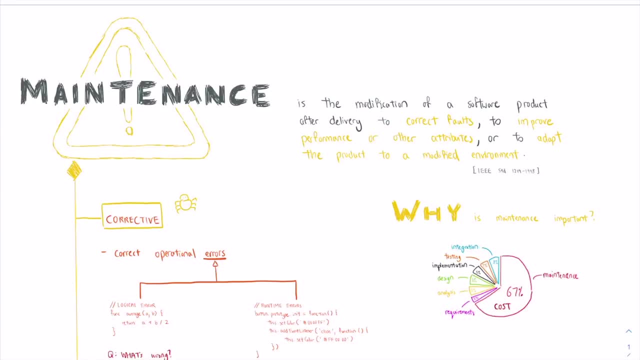 At this stage, we have introduced most of the key processes in software engineering, regardless of whether you are primarily agile or waterfall based. So the last key process that we will cover here is maintenance. So let's start with a formal definition and according to IEEE standards. 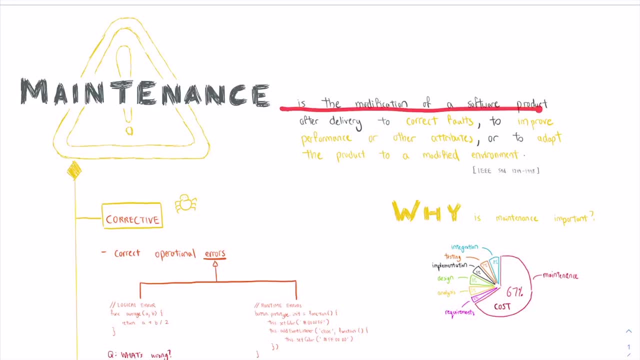 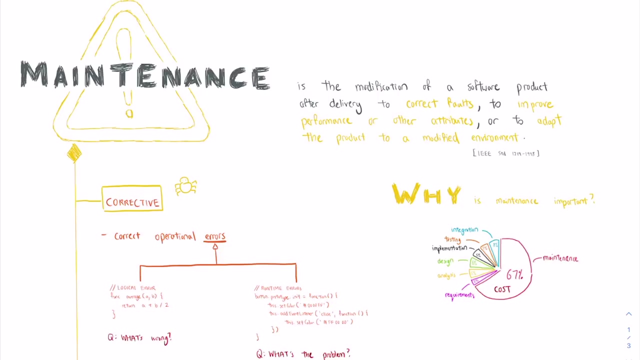 this is the formal definition. So maintenance is the modification of software product after delivery to correct faults, improve performance or other attributes or to adapt the product to a modified environment. With this definition we can basically determine the constituents of maintenance which can be seen in this side, over here on the left side. 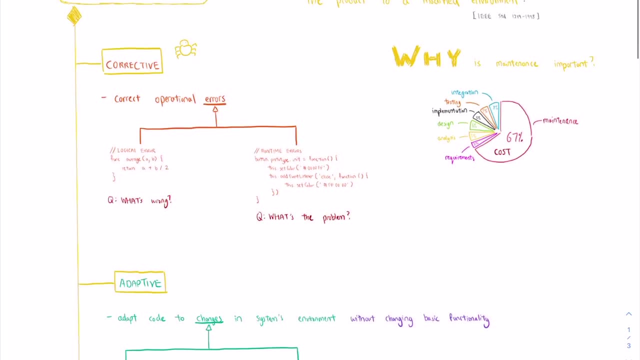 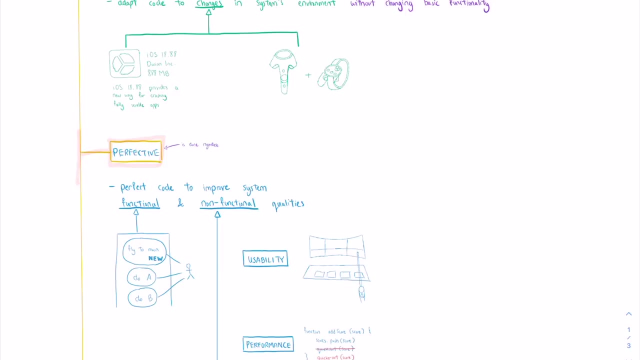 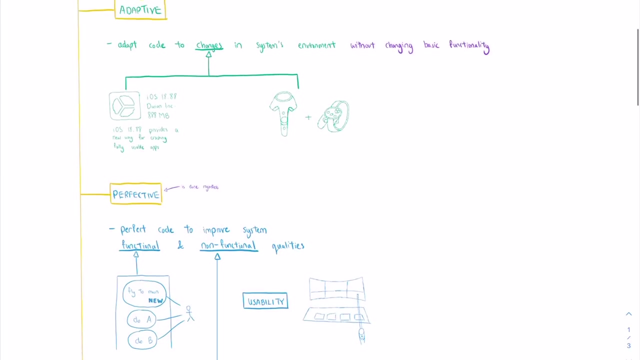 The first one being corrective maintenance, the second one is adaptive maintenance and the third one that is included in this maintenance process is perfective maintenance. So before we delve a bit deeper into this constituents of maintenance, let's establish the main reason why maintenance. 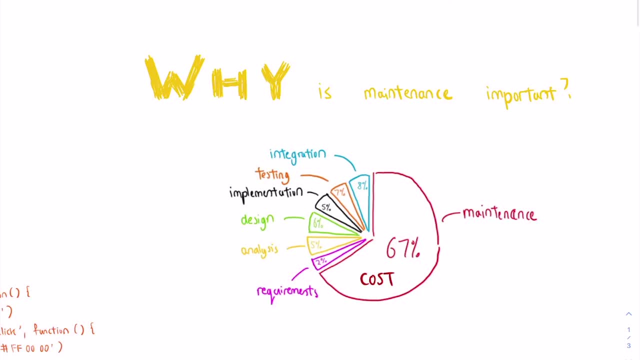 is important. So we see this graph over here or this pie chart over here, where the percentages basically represent the cost. as usual, Always, some of the priorities that we set are often related to the cost of what it takes to build this software, And cost, as we know, is also related to the effort, as you guys have practiced. 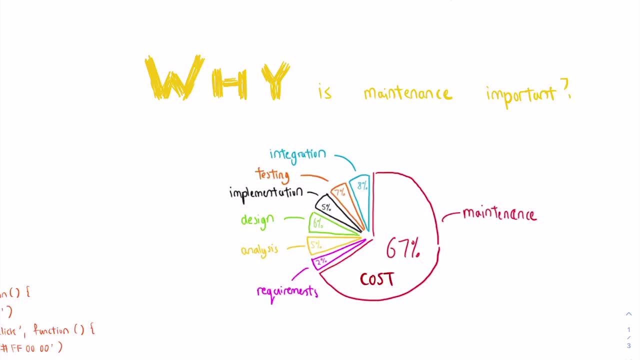 effort estimation in the early parts of this module. So whether cost or effort, I mean, they can be treated as synonymous right here. So we can see that this is a typical representation of maintenance. Of course, the exact numbers over here is not the most important thing. 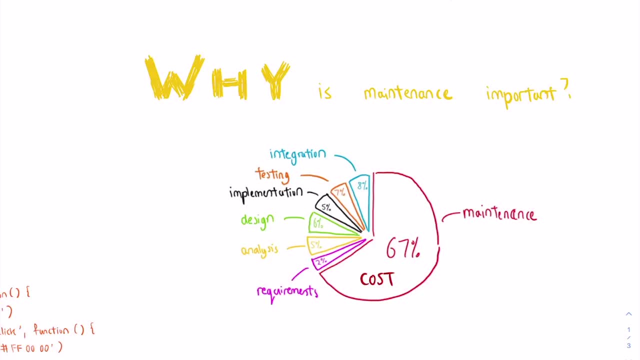 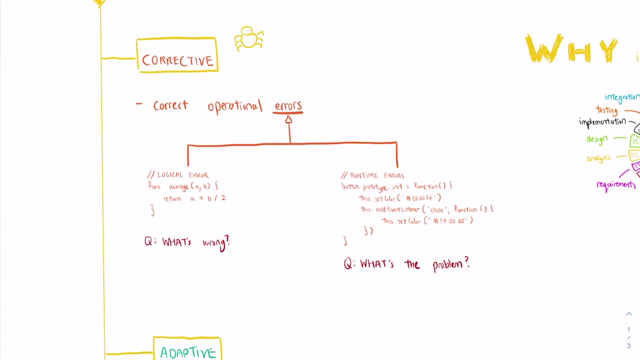 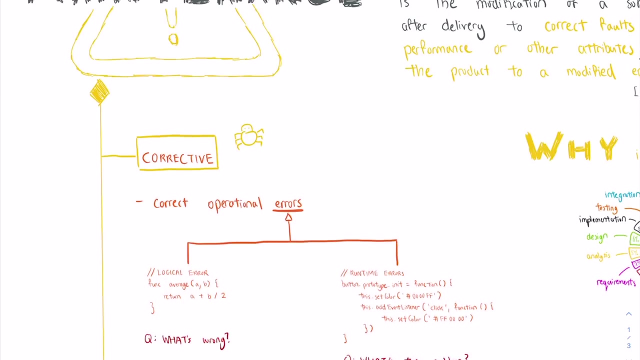 But basically this enables us to know that maintenance takes up the most amount of effort and, in turn, it is taking the most amount of cost in any software project. With this, I guess this would be an important aspect of software engineering that we should spend a lot more time in. So let's just go into each one of these components of maintenance. 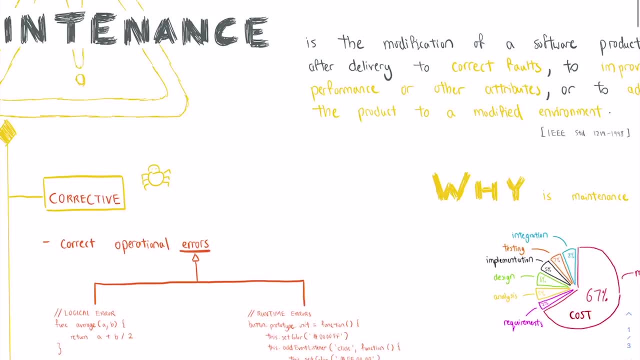 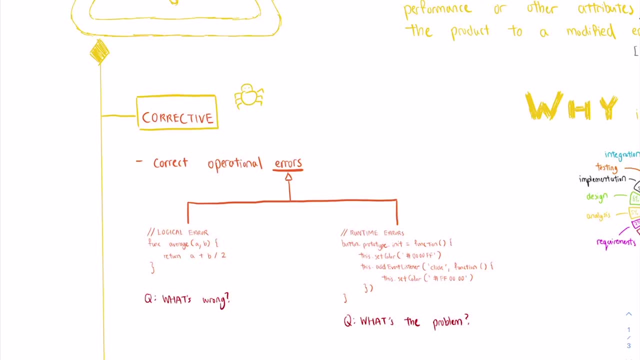 So the first one is corrective and, as indicated already in the definition, one of the key things that you will do in maintenance operations is to correct errors, And what sort of errors I mean. it's not that you're going to be solving any sort of problems with your software, but because it is. 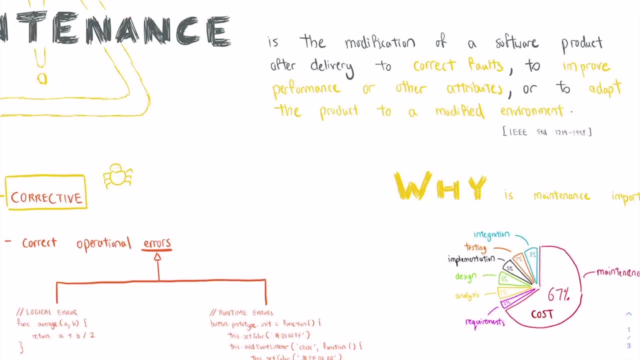 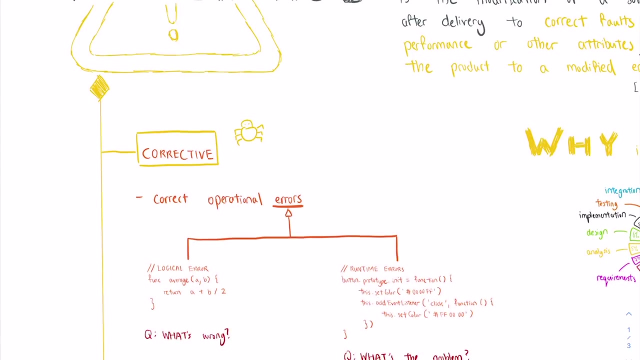 already delivered. maintenance is this term that basically refers to, after you deliver something, what continues to happen with your involvement with this software project. So, since it is already delivered, we can sort of assume that the errors that we are talking about is going to be operating errors. So that's why I put this over here. but the main point here is: 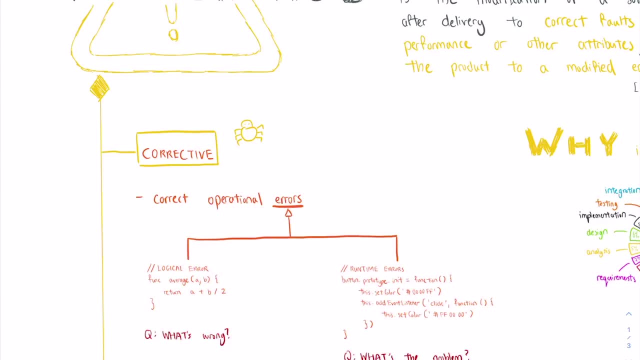 in general, these errors are going to consist of operational errors, So this is why I wrote this over here. In general it can be sort of related if we think about programming itself, Not so much of compile time errors. I assume that those have already been addressed since. 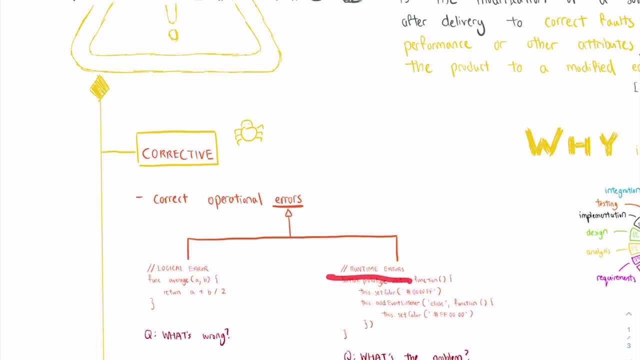 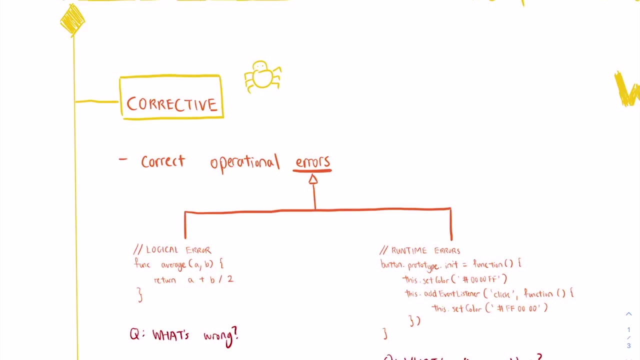 we are in production and when we talk about maintenance, It's more about operational errors. example over here, For example, this shows an average function on the left side over here and you can see pretty much that, due to whatever reason, carelessness which happens to all of us during intense 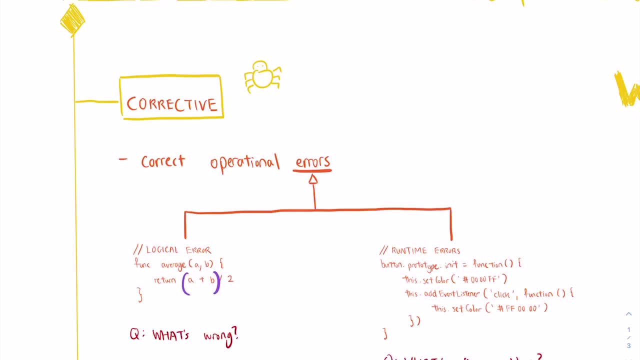 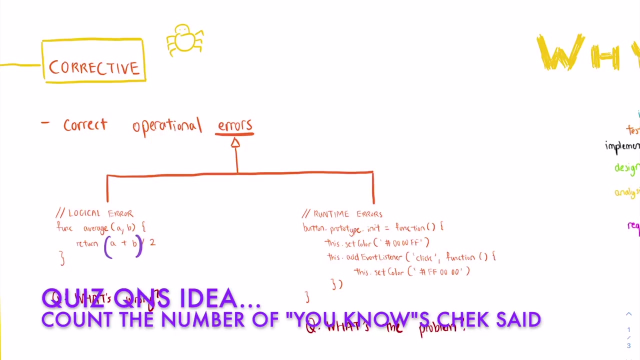 bouts of coding that we forget about the bracket and will produce the wrong answer. So this, as we know, is known as a logical error. Similarly, here, this is not really a logical error, but it is still a form of runtime error and in general, there's so many different types of runtime error. 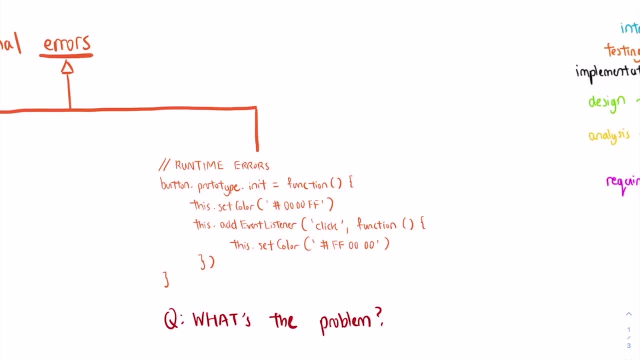 Like here. if you're not too familiar with JavaScript, you may think about JavaScript having the same kind of scope as normal JavaScript, Like general programming, general-purpose programming languages, But in fact it has some of its nuances which easily trips some of us up, like 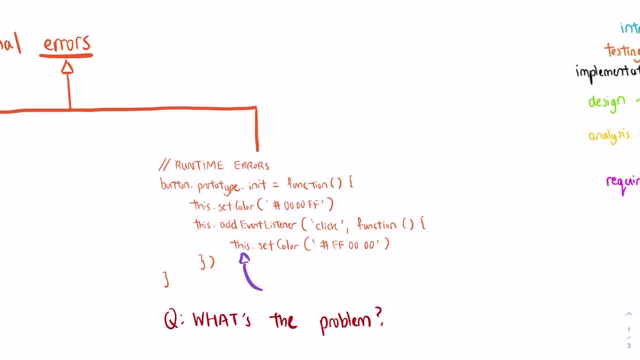 this over here. So this function it's pretty common that in your website you want to have. when somebody clicks on a button you would set a color. sorry, not click on a button, but this button. basically you would first set a certain color. 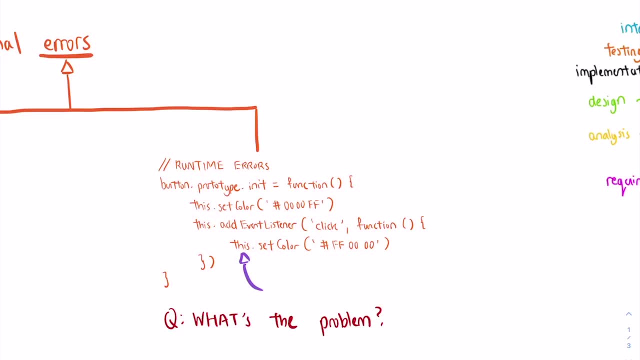 as the basic color. But when you implement a button, definitely you would implement some sort of a callback function based on certain events, Like the click event. When you click, this code wants to set the color of this button as another color, But the problem is: 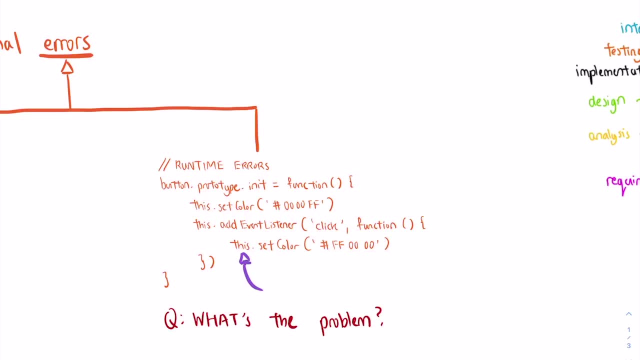 that in Java this scope is a bit of a different thing, So this is actually a the wrong scope. We've not delved into further details. of course, you can go and google what is wrong with this, and this will cause a runtime error because it cannot. 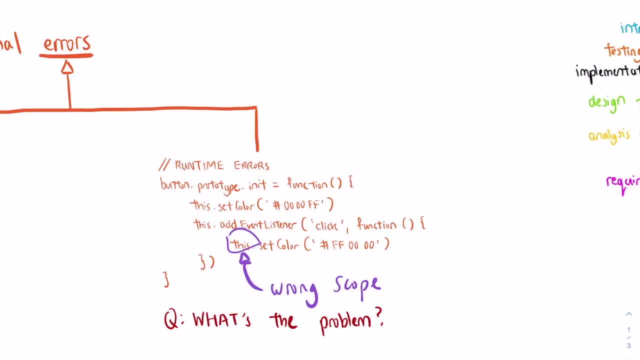 find the object that this is referring to that has the setColor function. Other types of errors may be also like infinite loops or memory leaks. All these things are common runtime errors which in the minor sense may not crash but produce strange behavior like intense lags in your software, or it may just cause. 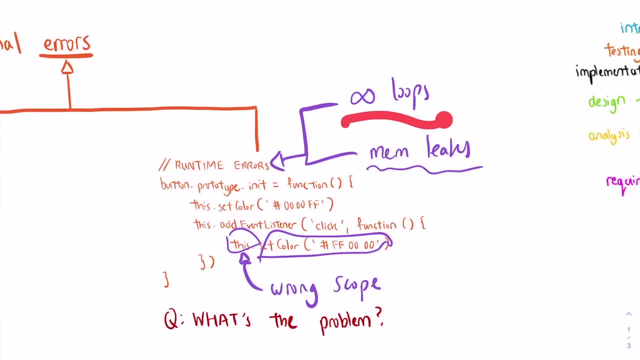 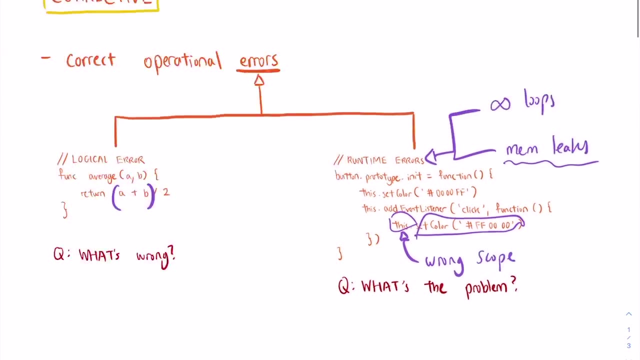 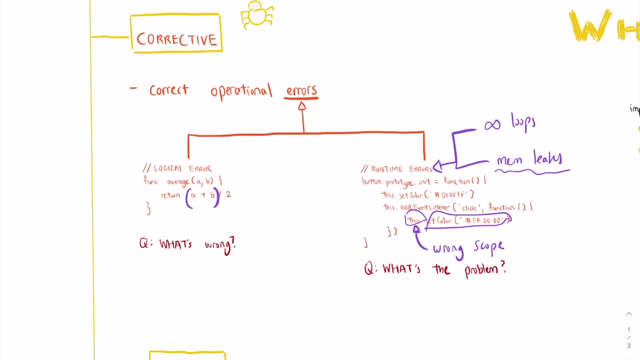 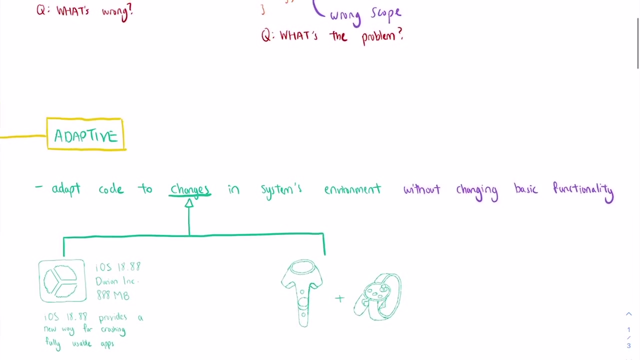 your software to crash or run forever. So all these behaviors that really you want to avoid. We need to correct all of these things and in general this is classed under corrective maintenance. The second portion of maintenance is called adaptive maintenance. It is basically required because of the environment that your system or your software is in. If you have a system that is not correct, you may not be able to fix it. The second portion of maintenance is called adaptive maintenance and it is basically required because of the environment that your system or your software is in, The environment that your system or your software is in. 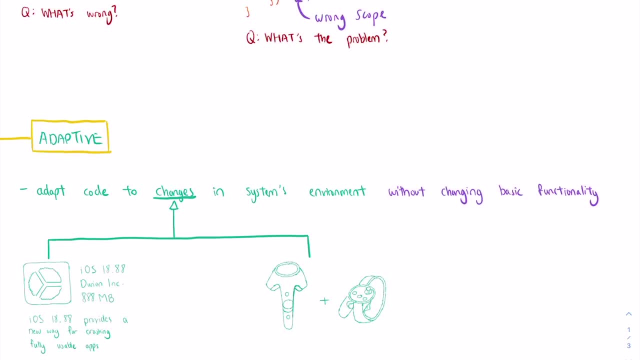 The environment that this production software definitely is dynamic. The environment that this production software definitely is dynamic. So conforming to this environment changes environment as we know, in our real human environment, it changes every single second. This is a core part of things that we 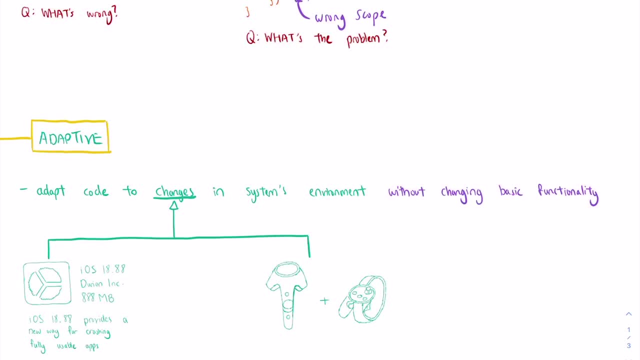 whether as humans or whether we are coding, we need to adapt to. That's why this is known as adaptive maintenance. That's why this is known as adaptive maintenance. So the examples here. one of the things that I wrote over here is that 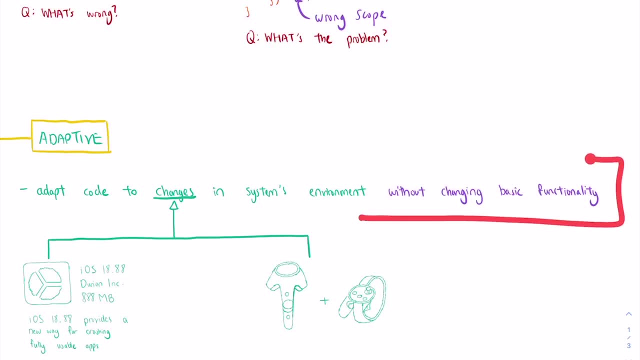 you are trying to maintain the code without changing basic functionality, Because here we're in maintenance phase and what we want to do is that we want this at least for this type of maintenance. is that actually we are not trying to change functionality or anything, It's just that we want to maintain the same functionality. 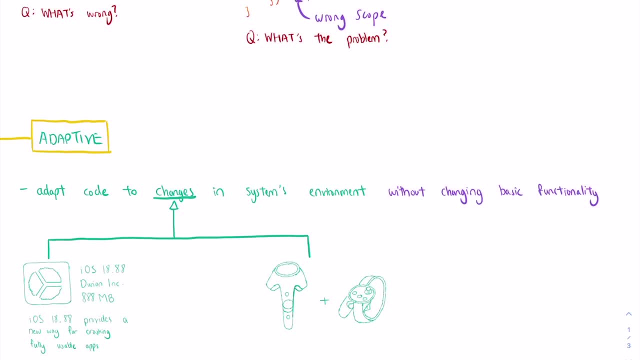 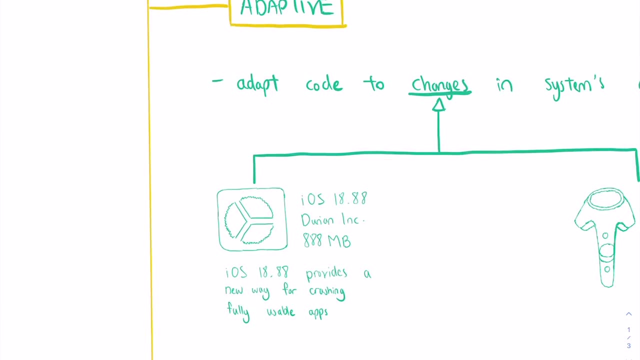 the same functionality to work. when our environment changes, For example, the most common change that we will encounter is the operating system, Because most software relies on some form of operating system to run the software, Like in this case, if iOS comes up with a new version, it's pretty common that 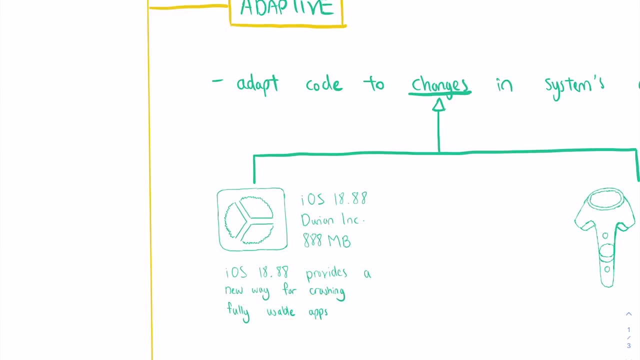 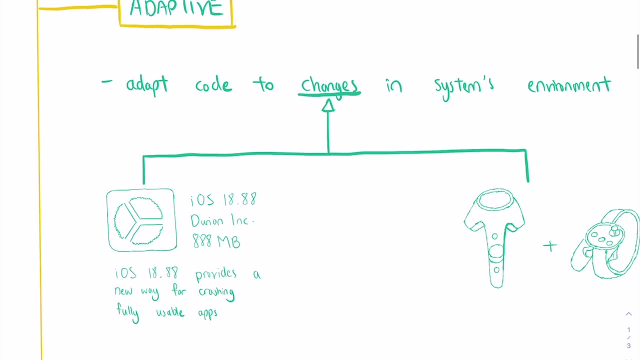 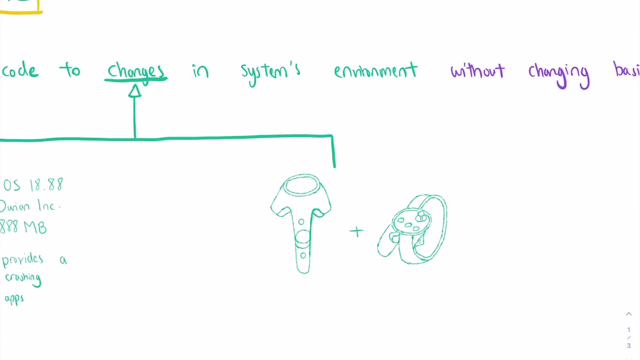 your app may not function in the way that you have expected. It is the cause of most curse words against the big tech companies. Other changes other than software: the OS that your app resides on, which constantly updates because the OS and the big tech companies that runs the OS on the devices that they come up with. 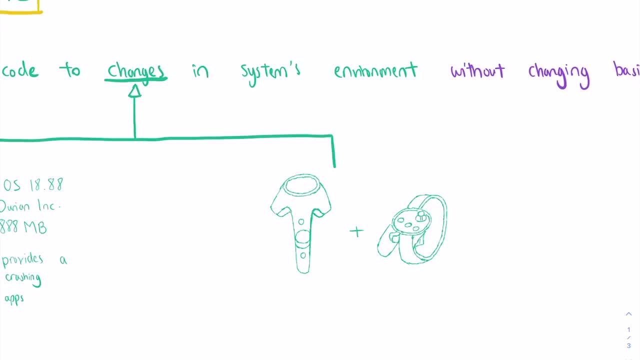 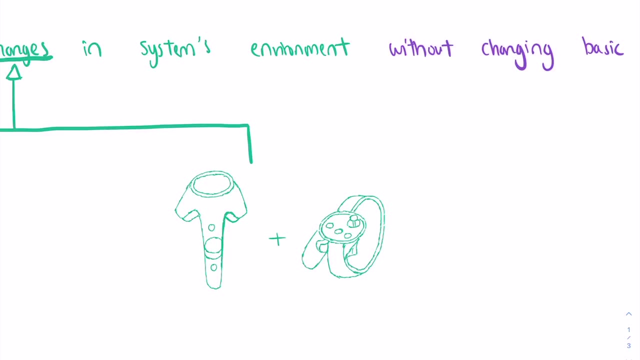 they always want to improve as well, So we need to go along with that. Other than software, hardware is also something that's pretty common. Examples here is just in terms of a VR example, For example, new versions of the VR controllers that your app resides on, like the Oculus Quest. 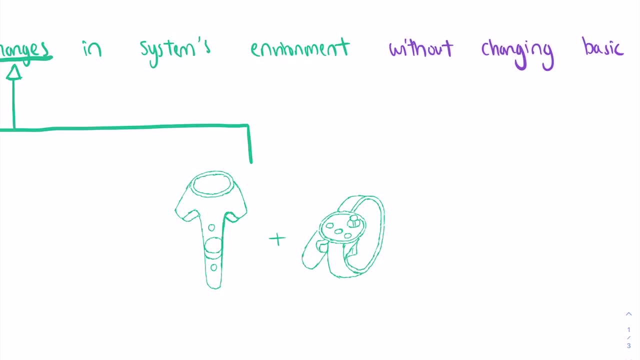 next version the controller has a new functionality or has a changed functionality, then you're sort of obliged to support, Even if it is some new thing that doesn't really affect you. it comes up with a new controller and you need to change your code to conform to the way it works. 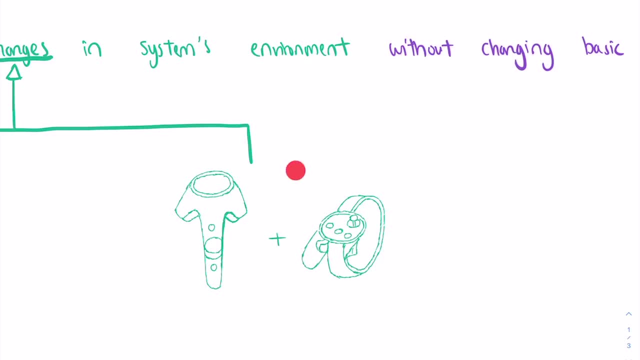 You would sort of need to do that, otherwise you will lose users who are on the new controllers, And other examples might be just the fact that the new flagship phones are being introduced, whether with or without the notch on top. All these things. 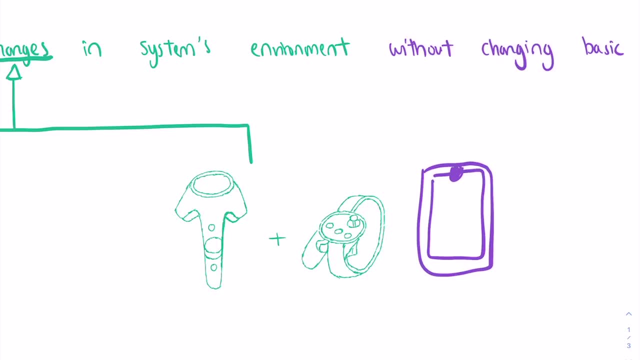 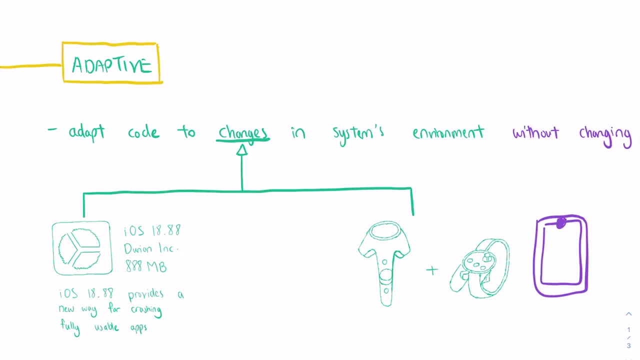 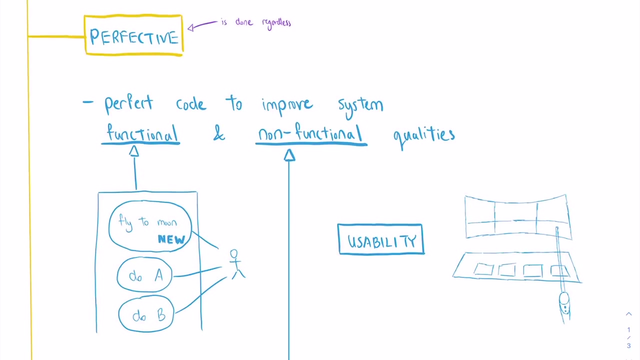 So if you have a new controller, you might need to change your code to conform to the way it works, All these things that you need to conform to whenever the hardware changes. So these things are known as adaptive maintenance, The third part here. actually, there's a fourth part. 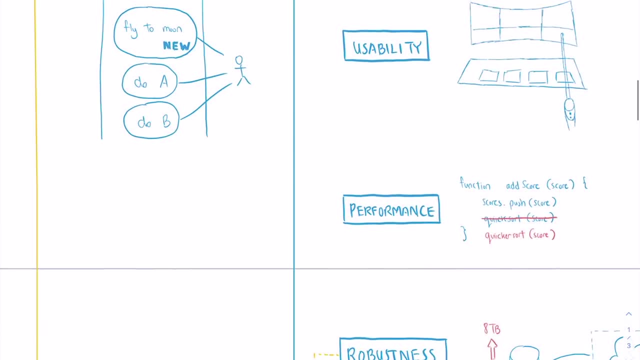 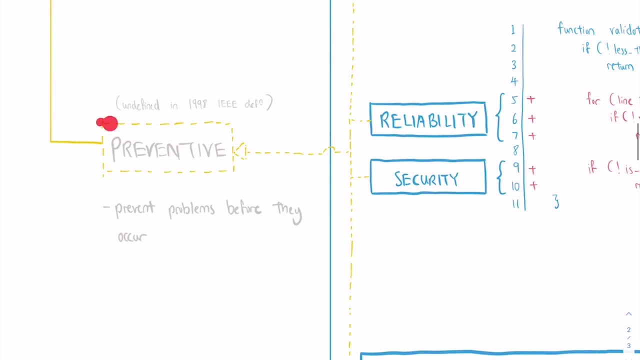 But this preventive maintenance is sort of subsumed into perfective maintenance. In other words, this preventive maintenance is sort of subsumed into perfective maintenance. IEEE used to have this, but as years go by, the recent definition doesn't really explicitly. 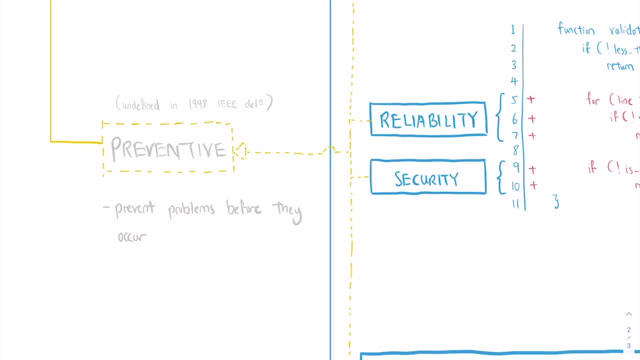 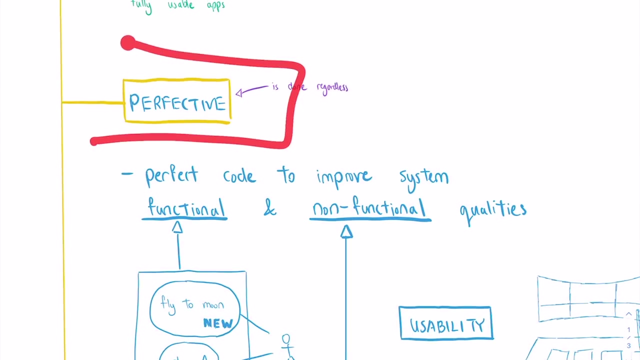 mention preventive maintenance, Although when you read online some texts still stick to this word- to differentiate the types of maintenance that you do that prevent problems before they occur, versus other types of perfective maintenance that you try to improve the system's functional and non-functional qualities. Although this preventive 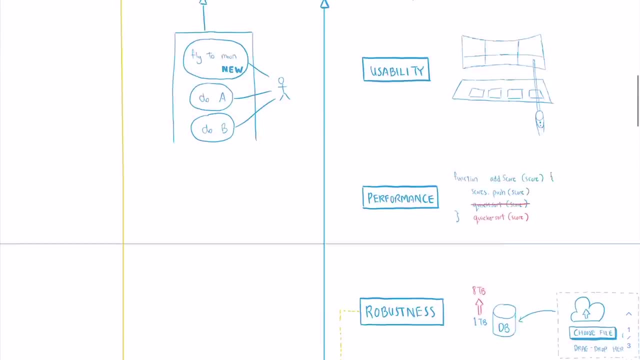 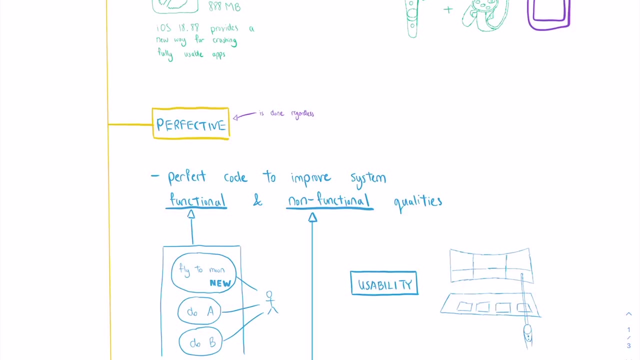 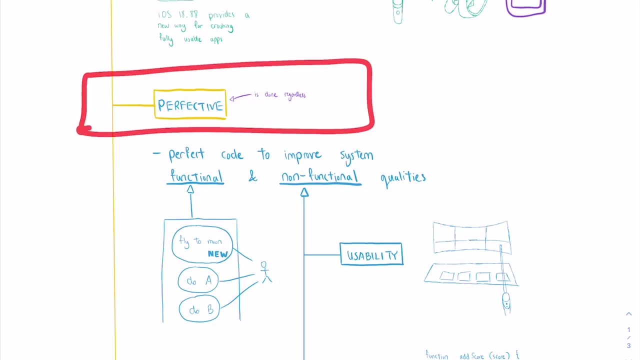 maintenance operations that you do may also be classed under this definition. Just a minor distinction over there. whether you want to have this distinction or you don't Need to understand this distinction is up to you. This perfective maintenance is actually huge because it encompasses all improvements that 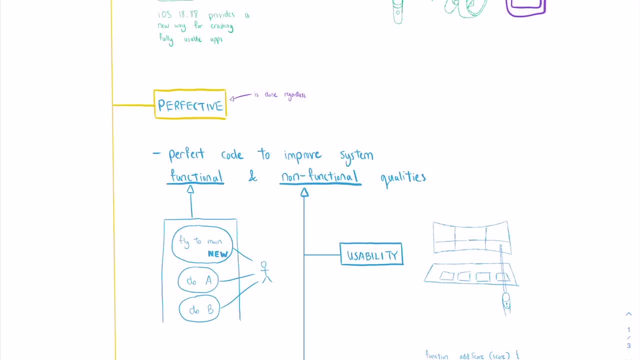 you can do to your app or system. As the name implies, you're trying to perfect your code to improve the system's functional as well as non-functional qualities, For perfective maintenance of functional qualities. it is pretty straightforward to understand because it is basically adding use cases and working on. 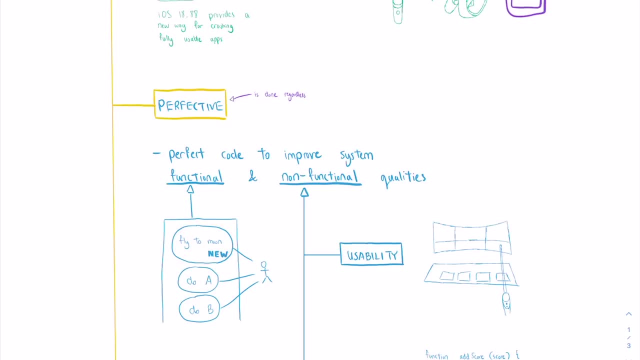 them. This is called functional perfective maintenance. For example, it's running version. during the maintenance phase, Your company or your team- if this is an app that belongs to your company's product- you decide that this new feature would really add to the usefulness of. 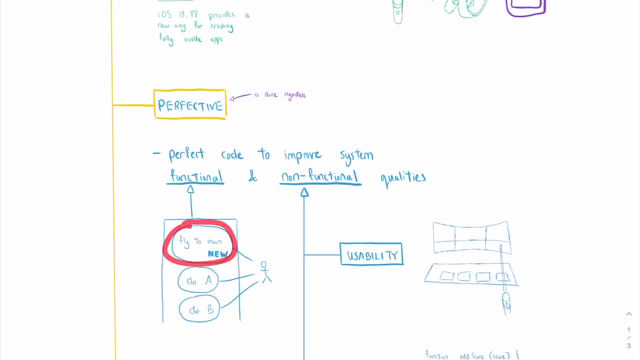 whatever you're offering the app or system- This is very important because you're trying to improve- is in this app, so you need to add this and work on it during the maintenance phase. so this is functional quality perfective maintenance. for non functional quality: well, it is a huge rabbit hole, as you can see in this long 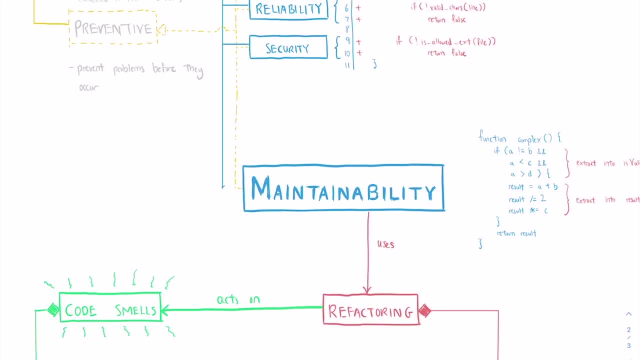 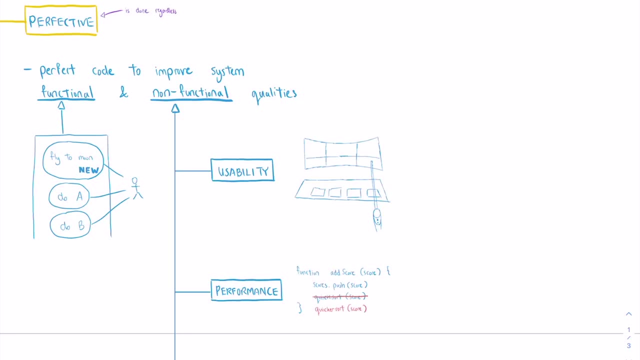 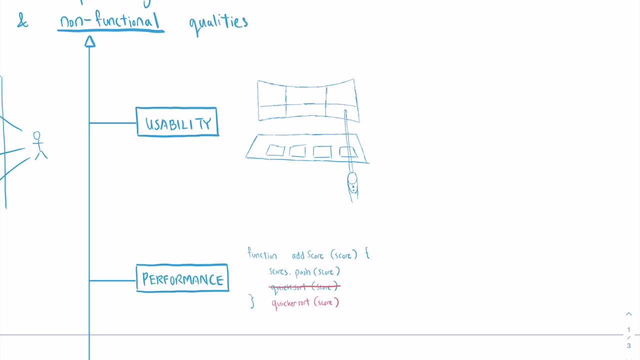 list of different things. sorry, that's missing one line here. okay, long list of different things that can be a type of non functional quality. okay, which includes the usual suspects of software quality, right as we know, in non-functional requirements okay, like, for example, usability in general. improving usability of various aspects of your app is a constant endeavor, and 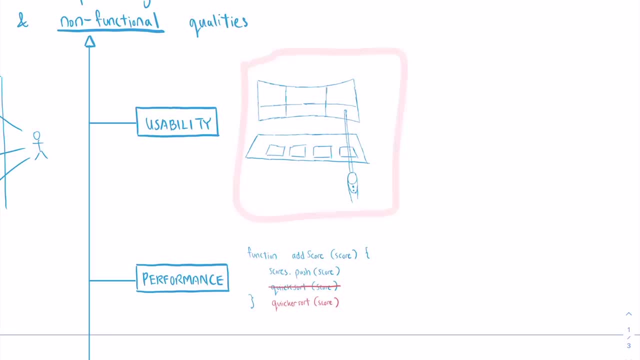 this example of a VR interface may be a bit more extreme. okay, as it is a big open research problem with no clear guidance. so you need to constantly, you know, iterate, create different types of interfaces- curved flat and so on, 3d interface- and then test on users and then improve this. 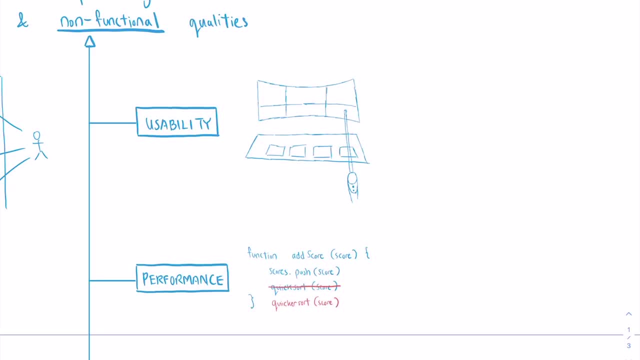 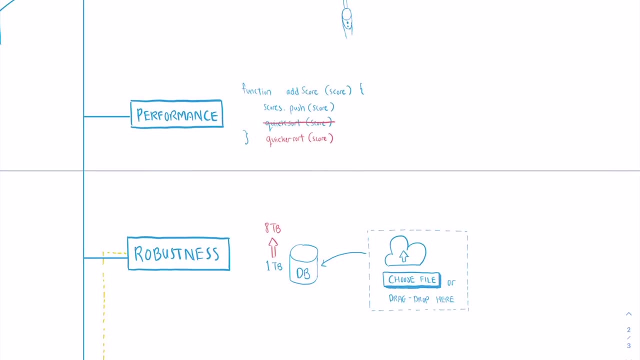 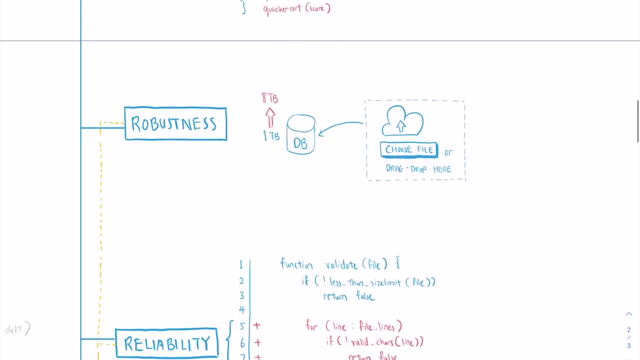 usability aspect of you know this type of interfaces and for performance, right. similarly, you know this is like a constant pursuit of you know better speed and lower memory, okay, like in this case, improving the sorting algorithm in your code, all right. other examples of the common you know: robustness is, you know, basically trying to improve the stability of your system. 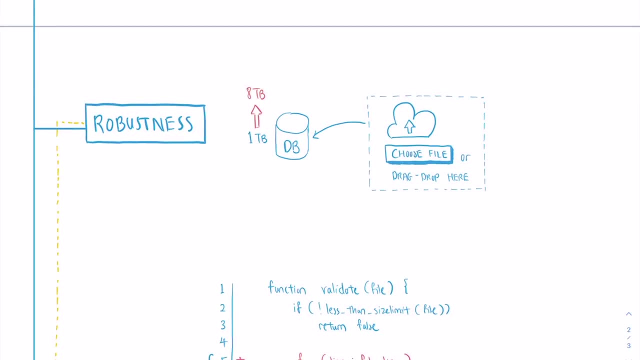 by enhancing its ability to handle special or stressful situations like this example over here. increasing our back-end database drives size okay, so that our uploader interface will not stall right in the user space when there is an abnormally large number of concurrent users who. 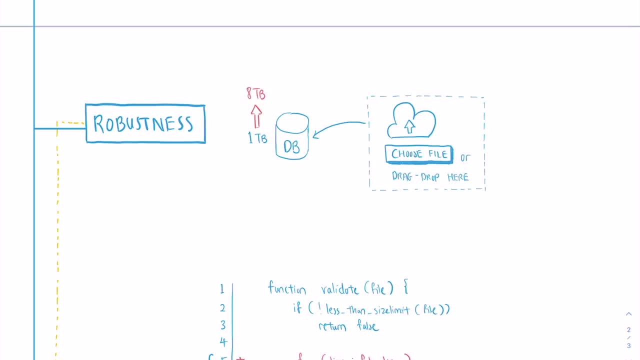 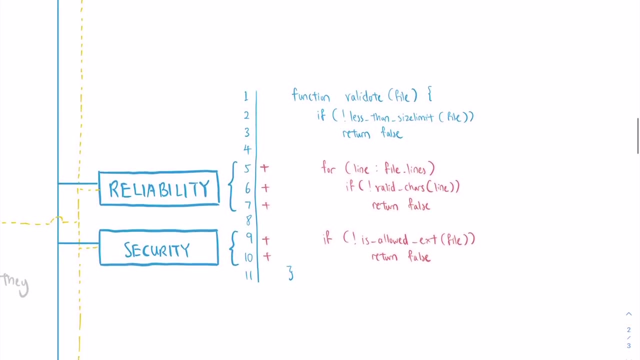 are trying to upload in the system. okay, so this actually improves the stability to handle special situations like that. okay, so that is robustness. Other common terms of software quality are also examples over here. you know like reliability basically refers to preventing. 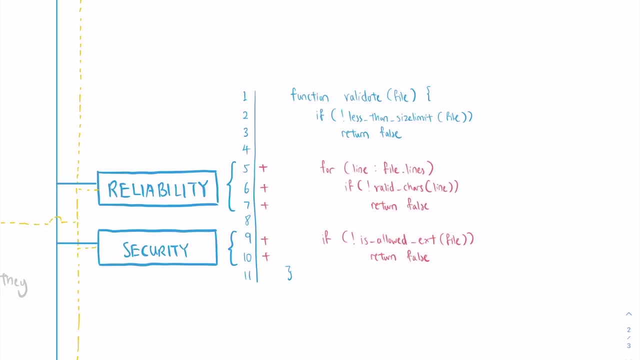 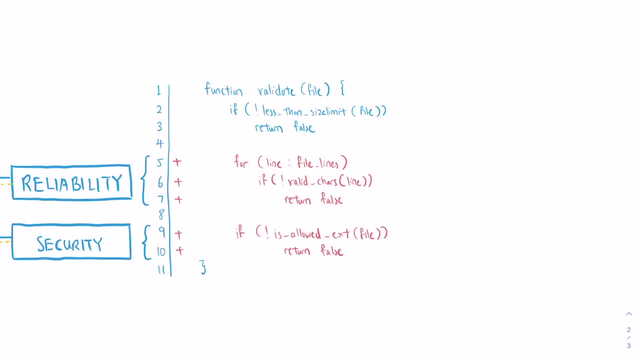 crashes, uh, by catering to more types of situations that you expect, you know like, adding this extra check over here would allow you to prevent your app from, you know, exhibiting bad behavior by, you know, catering to more types of situations. okay, making it more reliable. 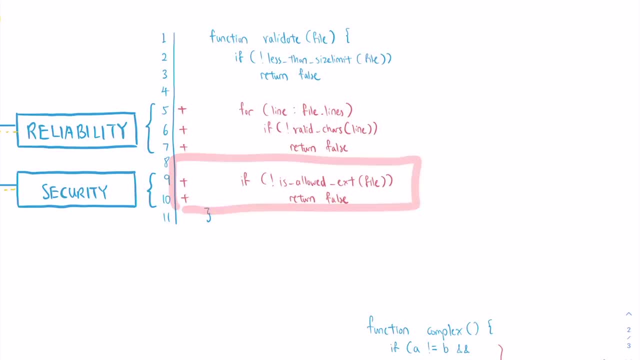 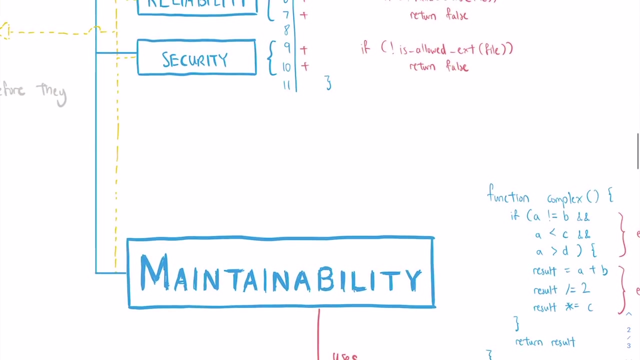 And security. you know, this is just an extremely trivial example of improving security by adding a preventive check against possibly malicious files. all right, Then we have this um last part over here, which is maintainability. okay, Our last type of. 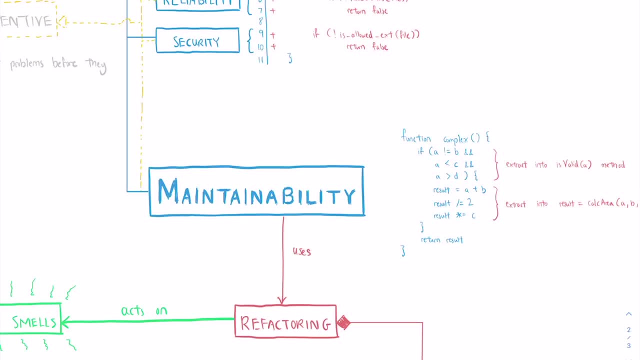 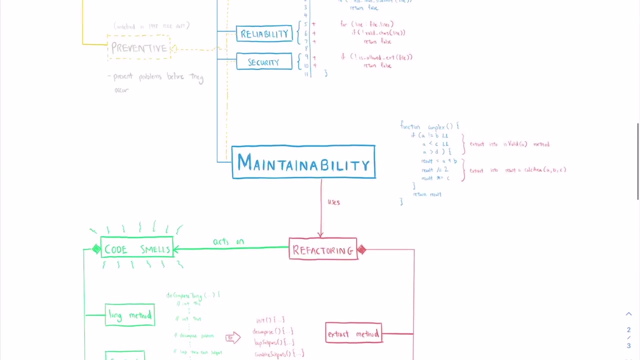 non-functional quality that you may want to do in your maintenance phase and as this word implies, okay, maintainability, you know, maintenance okay matches maintenance really well, which is why this aspect is, you know, the largest rabbit hole. What does this mean? I guess most of you have come. 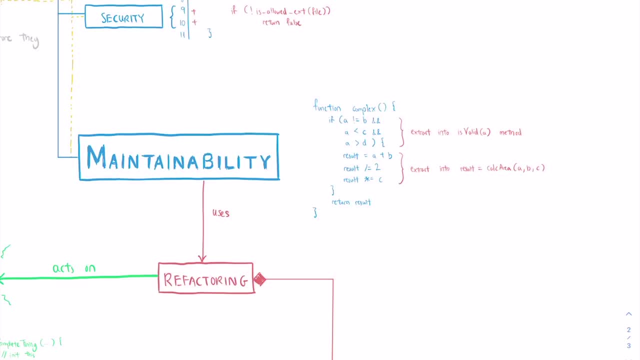 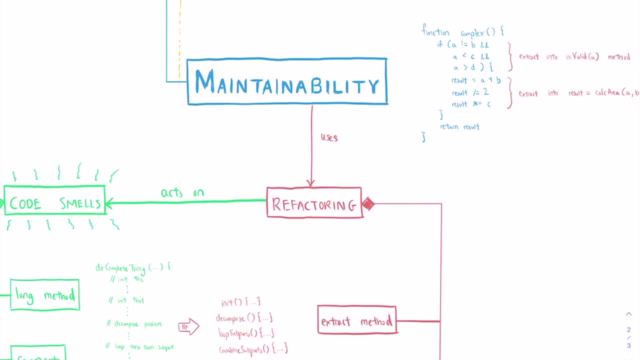 across this word when you are trying to establish good coding practices, In a code review, for example. maintainability is a big goal that a code reviewer tries to establish Sometimes. it may be often overlooked this non-functional quality called maintainability, because it's. 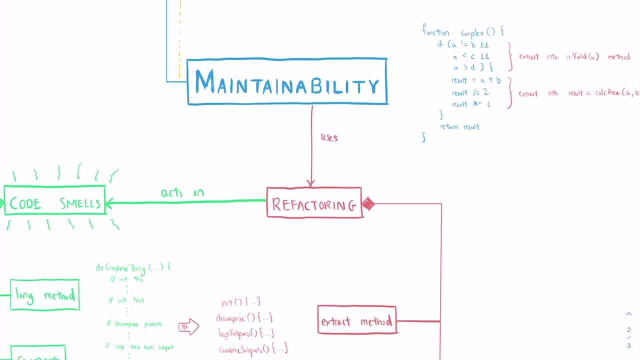 just so broad, sometimes a bit subjective. it depends a lot on your team's practices and so on, But there are many general good practices that all teams would want to look at and possibly customize for your own applications. It may not look like having better code it. 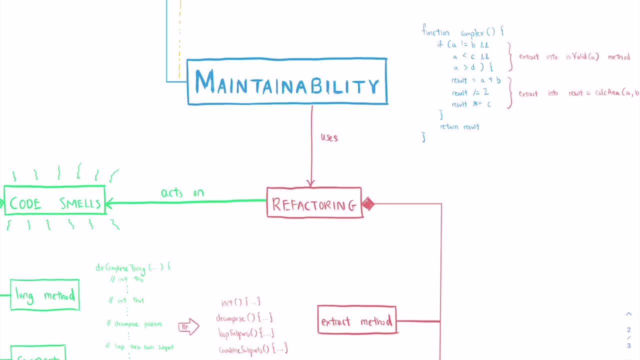 may not look like it directly enhances your product quality, but it actually does, and in a big way. It may not look like it directly enhances your product quality, but it actually does, and in a big way. If your code is more maintainable, it means that more people can. 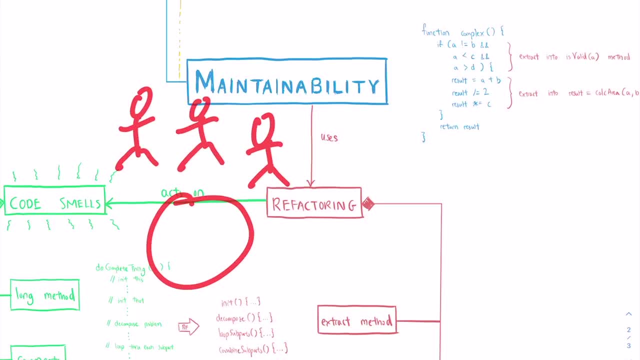 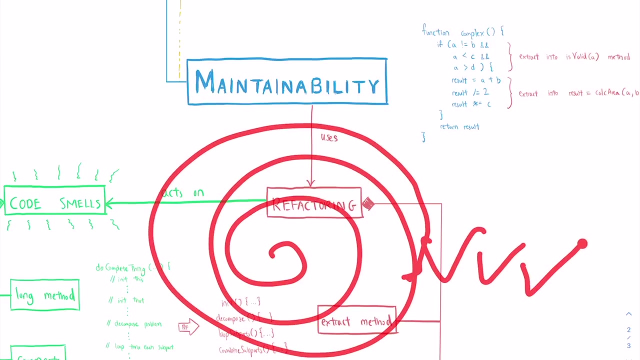 work on the same piece of code more easily, and we know that the key to good software is the ability to iterate well in development and slowly grind our way to good quality software, which is also why Agile has dominated most software projects- where it fits, of course. 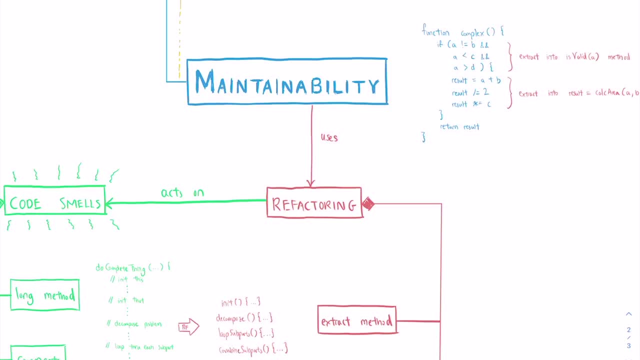 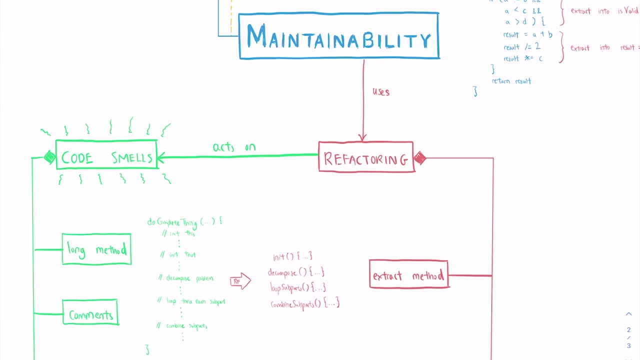 and where the stakeholders have the power to make this decision, for Agile processes to work. Okay. so, with that being said, let's look at what are the common things that we do when we look at maintainability as part of non-functional quality that we want. 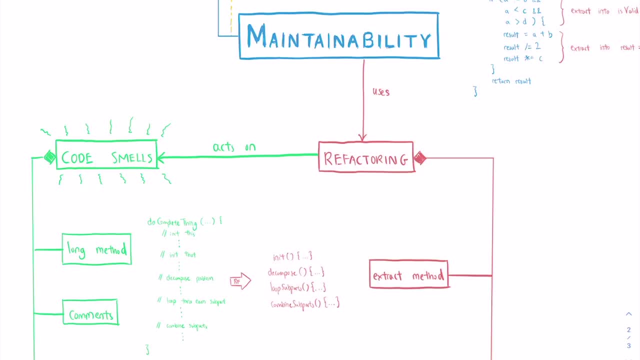 to improve during the maintenance phase. You can see that there's this matching two sites that we have here. You can see that there's this matching two sites that we have here. You can see that there's this matching two sites that we have here. 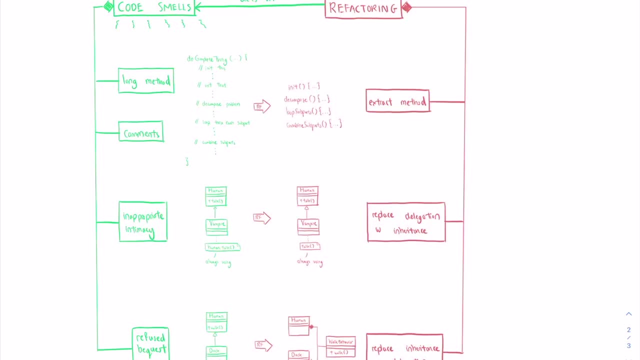 two sites that we have here, two sites that we have here, and so on. we have over here in terms of, you know, having code smells on one side, on the left side, as well as refactoring patterns on the right side. so what is this? this is basically, you know, as a software. 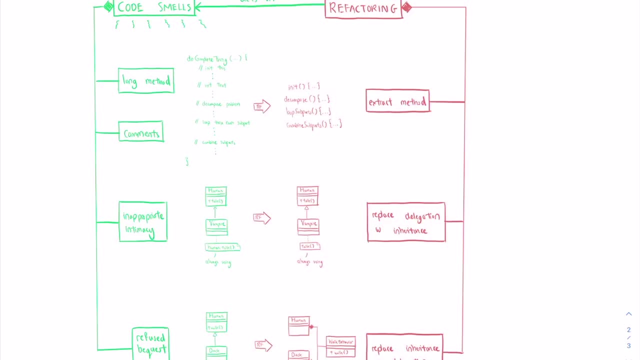 engineering. as a field, it matures naturally. people have documented the common pitfalls of code, normally commonly known as the code smells okay and consequently the common recipes you know that we are able to use to resolve them, and this is commonly known as refactoring. and here we are. 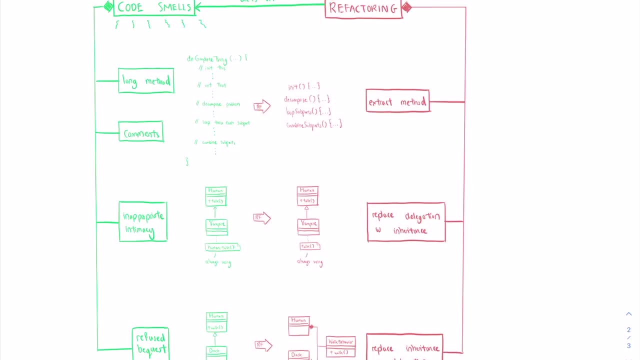 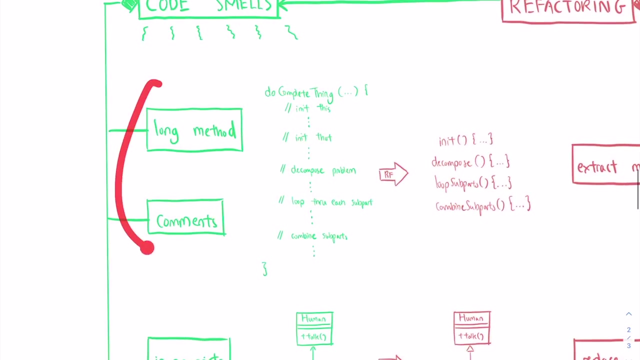 looking at refactoring patterns: okay, very similar to your design, a pattern kind of a concept, all right. so let's look at several examples over here here. this code over here- sorry, let me circle the right code here, so the code over here. here we can see the different types. there are a lot of different types of code. smells. 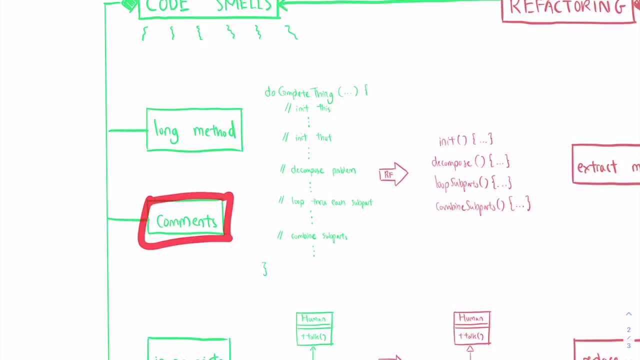 the first type is long method code smell and the second one is, you know, the comments code smell in general, but it is more aptly named as bad comments. you know, if we want to be more explicit about it, all right. so long method. as the name implies, it means that your method is too long, all right. 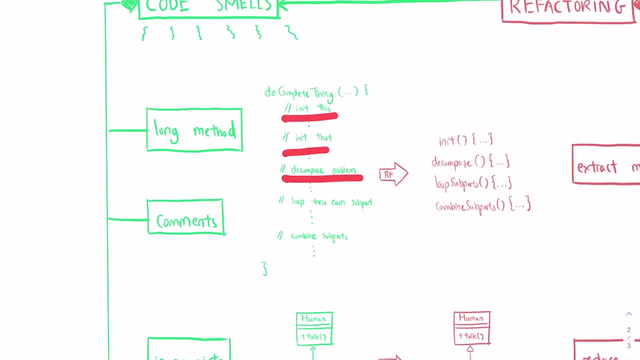 long you know too many different components, different responsibilities, in one single method At the same time. because it is so long, the coder probably needed to categorize this one single method into many different subparts. Once we see that, this is quite a red flag. 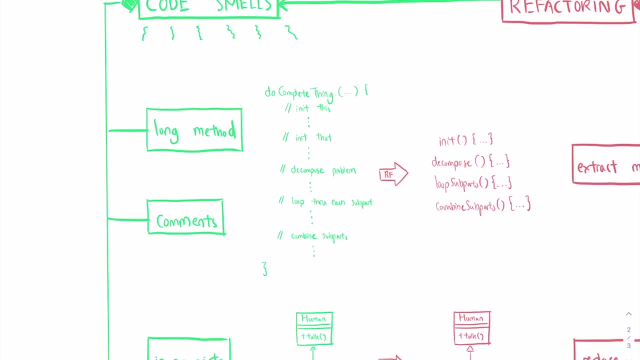 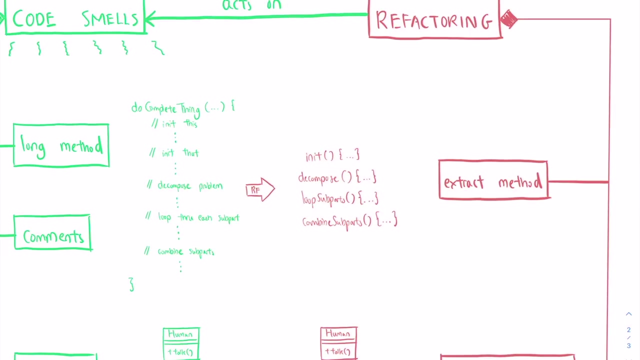 and it smells bad in the same terminology that this refactoring uses. Once you see this, you need so many comments section your stuff. it means that you are trying to do too many things in one long method. Naturally, the refactoring pattern is pretty. 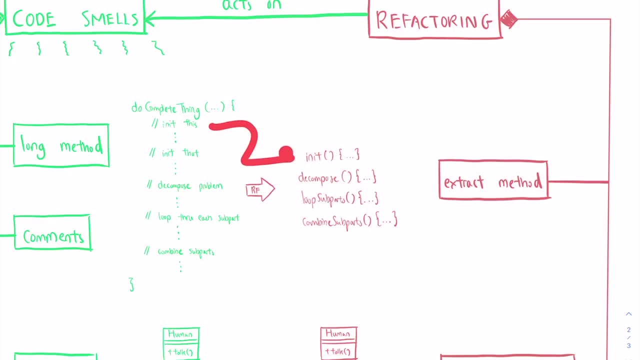 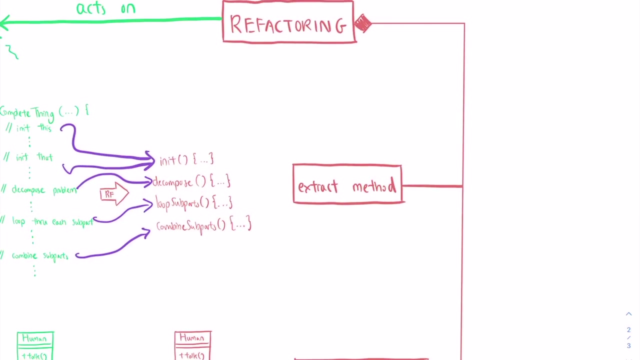 obvious To extract each one of these subtasks into its own. sorry, these two init. maybe just use something permanent: These two init functions into here, the decompose section into here, looping here and combining the subparts here. That would make your code much more maintainable, both in terms of the subcomponents. more understandable. 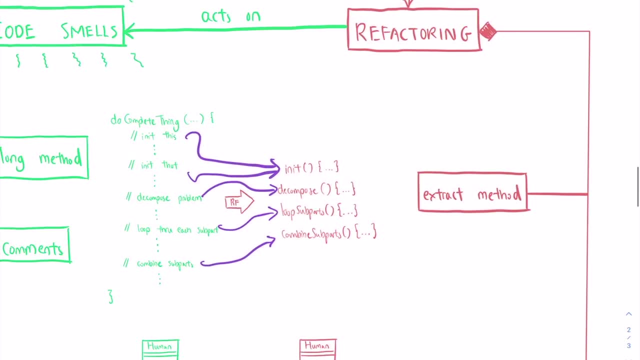 subparts and when you change a subpart there is no need to change one whole big function itself. For comments generally, we also do not want developers to spam inline comments or write long paragraphs inside the method itself. The internals of the method should be pretty. 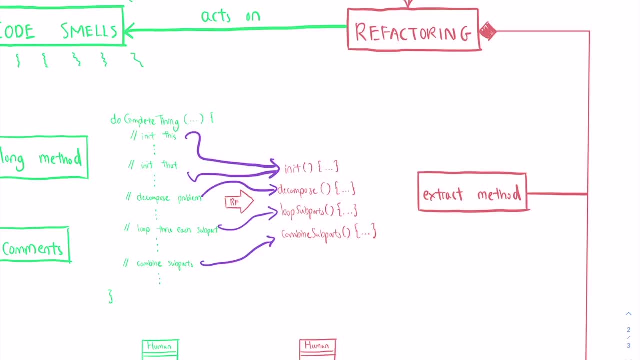 clean of comments and should ideally be self-documenting. I believe most of you know what that means: having your variable names nicely worded. It's not too hard to get all the comments in your own language. just think about it and see what you've learned. 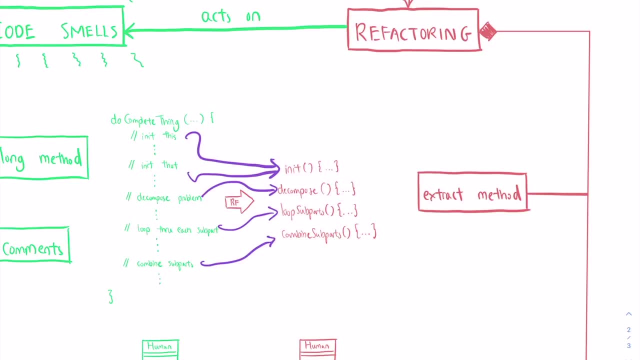 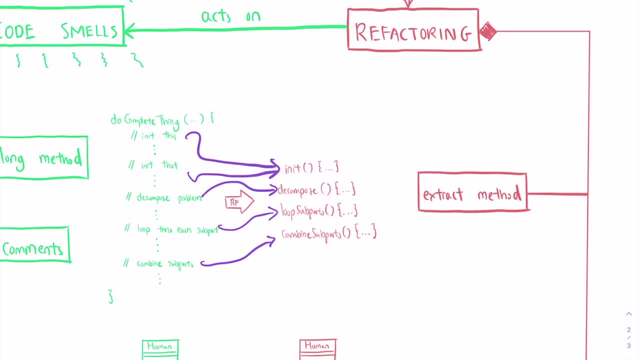 And if you need a lot of sectioning and explaining, I think probably you'd already smell something fishy. Now, speaking of comments generally, the main thing that we are looking for is the code haters, haters. Not code haters, but your function haters should be nicely documented, The entire. 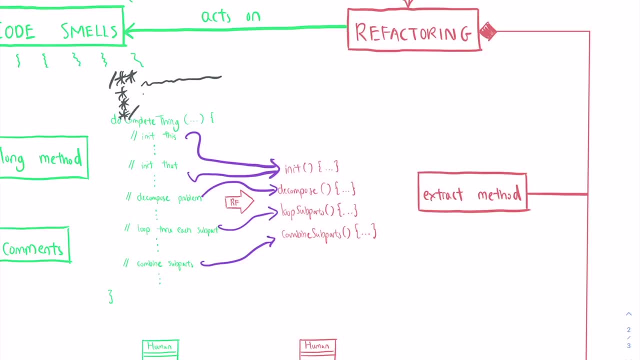 function should be able to be explained in a paragraph on top, with the proper input arguments- Not explanation- as well as the return argument properly explained. Another coder or yourself. after a year, when you look back at this function, you should be able to easily make out what this function does without looking deep into what is in. 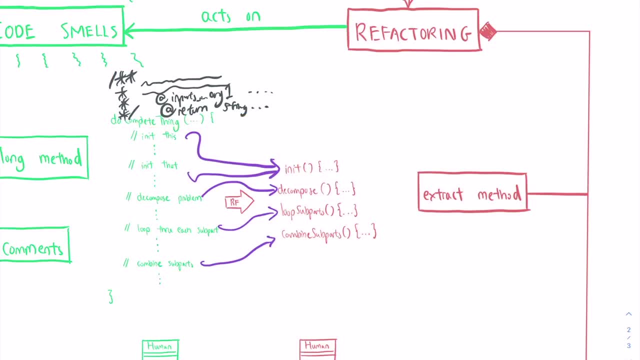 here. Just by reading what is here you should be able to make it out. And having such a big function, it's very difficult for you to have a, you know, a simple, concise paragraph like that. but once you have you know things separated into its constituents with very concise responsibilities, then you know you would have a. 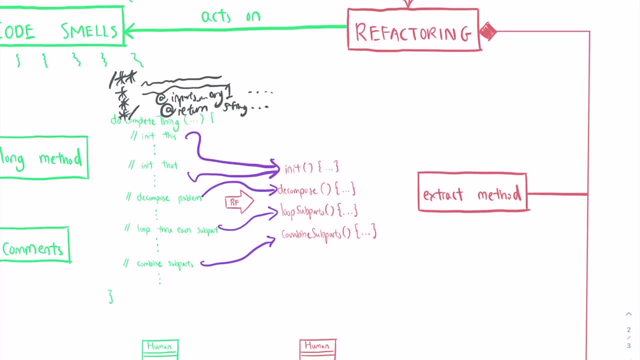 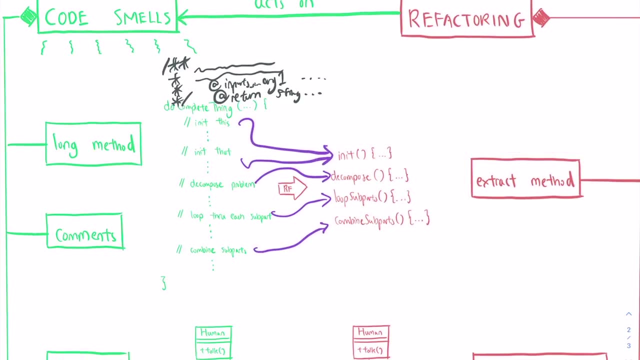 easier time, you know, making this section all right. so this is uh one example of a code smell and the refactoring pattern to deal with. this is called extract method and in fact in a lot of ides you would already find you know this feature uh inside there that you can just select. 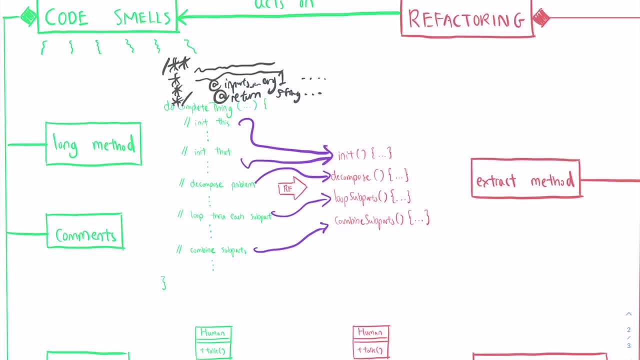 you know a certain section. you can just uh like, select this, and then you know, choose the extract method. okay, choose some extract method from your uh drop down menu. okay, and then you would be able to extract a function. yep, so refactoring, uh, you know the tools are already available. 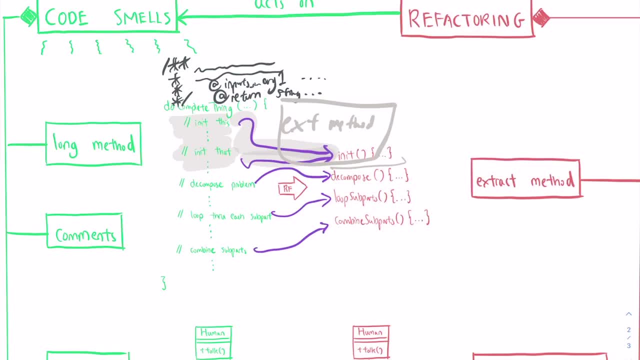 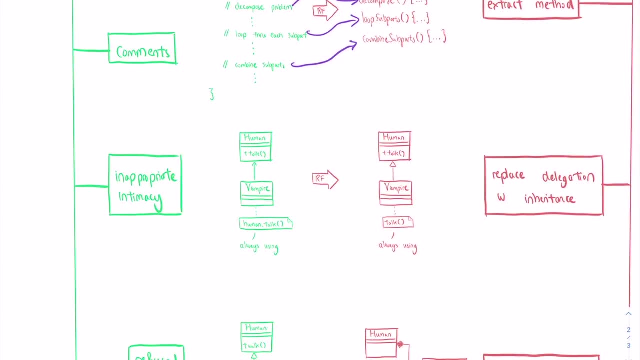 available, widely available, because these are some common things that we do in maintenance. okay, so the second example over here is: uh has a interesting name in inappropriate intimacy, all right. so, um, this is basically smelling of two classes being overly intimate. okay, uh, when they don't need to. okay, in real life we don't really interfere right with matters of the heart, okay. 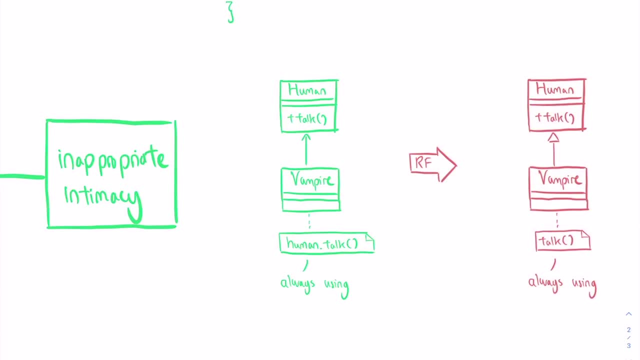 for other people, uh, that are maybe not within our family or whatever. okay, but even this is in our own code, okay, so we have to fix this. uh, inappropriate intimacy over here, all right, so, uh, what is happening here is that, you know, the vampire class, okay, only uses 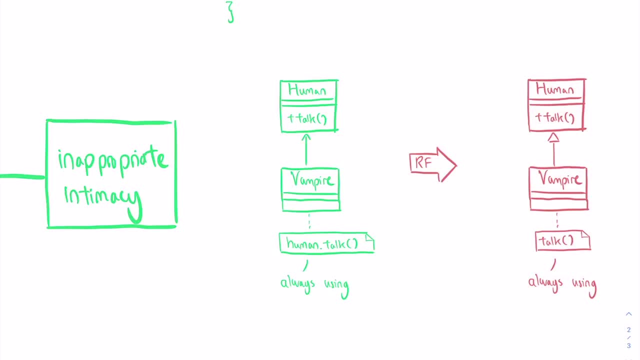 um, the human class to talk, okay, um, i mean, it seems to always uh, need this, this particular talk method, but the relationship is just, uh, uses all right, um, so it's like it's a closer relationship than stipulated in the relationship of the code. since, you know, it's so highly tied to this it needs. 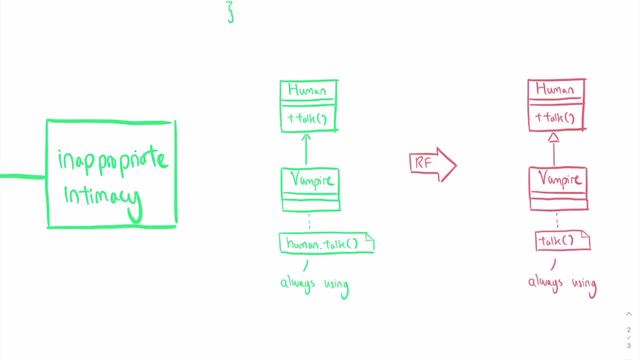 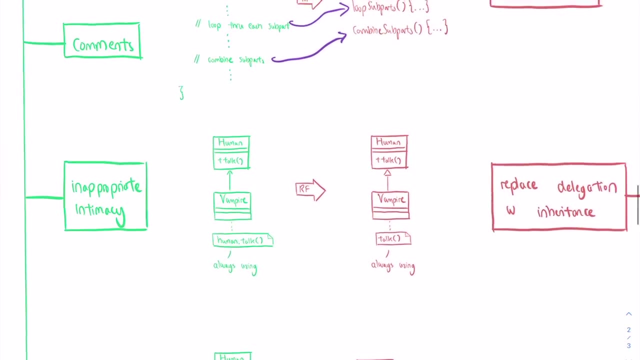 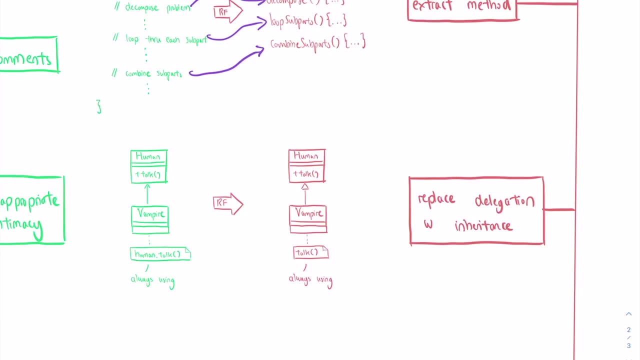 to function in order for a vampire to talk, okay. so therefore, um, the relationship should be closer. so, once we apply the refactoring pattern, uh, to fix this inappropriate intimacy, smell, okay, and the name of the pattern that should be applied is called: replace delegation with inheritance, okay, 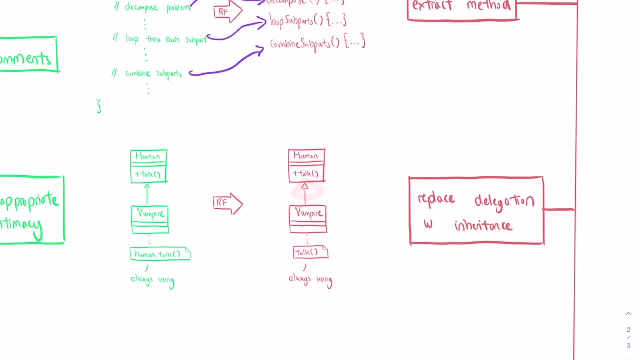 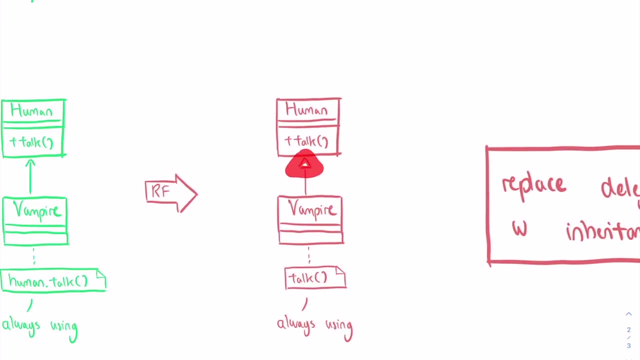 because this is like delegating and this is inheritance, all right. so, uh, there is a more intimate relationship there, so therefore, we need to uh, marry them okay by, you know, converting that relationship into something that is stronger, okay. so, really, a vampire is a type of, uh, human. 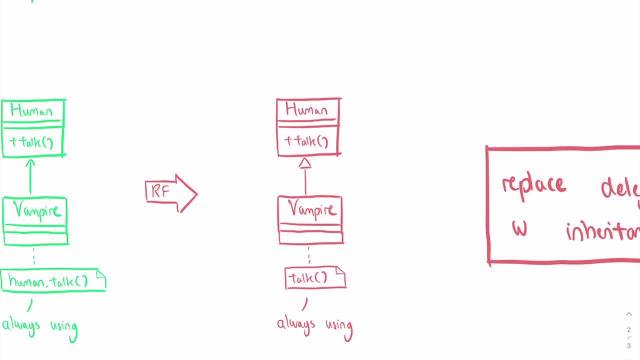 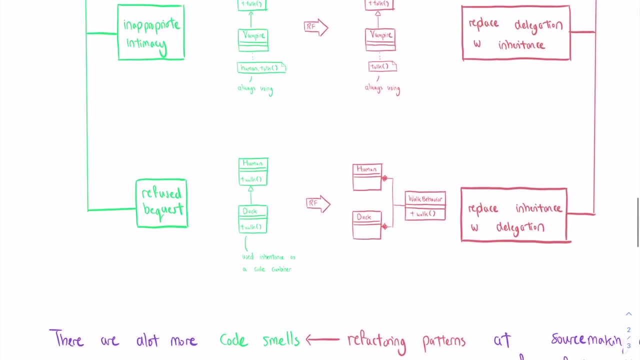 okay, so that you can directly use the top method over here. okay, so the last example is: uh, you know an even more funkier name, okay, um, you know, at first, when i first saw this name, i really have no idea. okay, until i look at the illustration and look at: 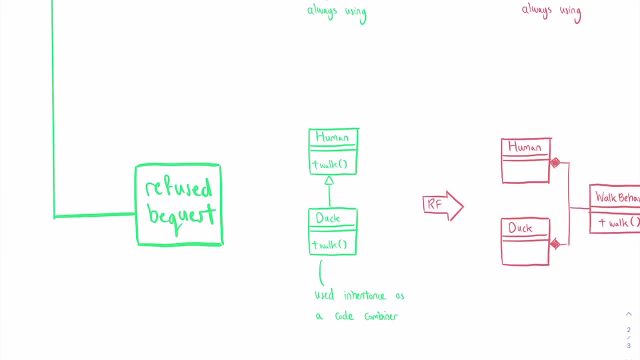 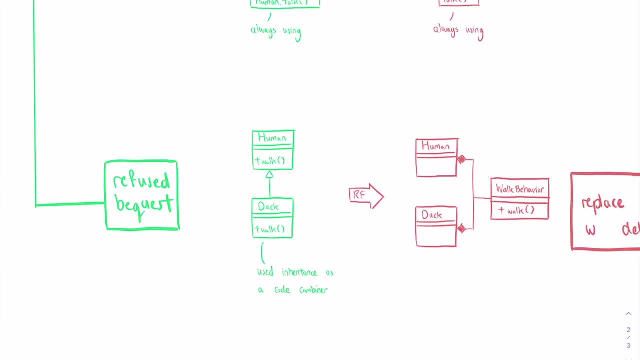 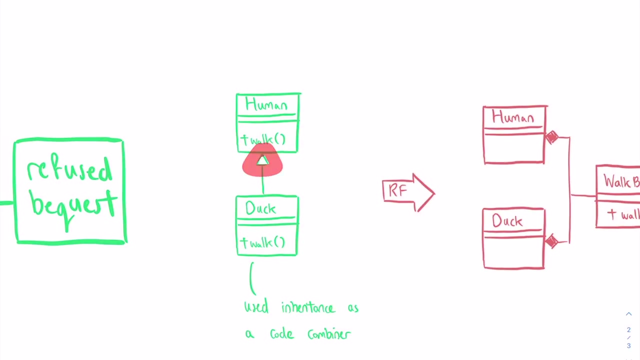 examples of what this actually means. okay, similarly, it is, uh, as trying to indicate that this code smells of a wrong relationship. okay, in a way, it's sort of the reverse kind of a problem that this is establishing a inheritance relationship. okay, um, where the duck okay is. 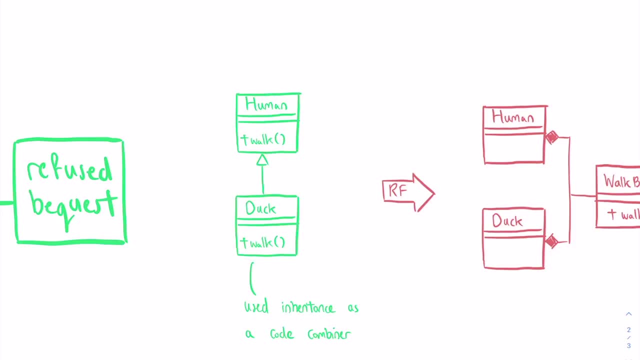 inheriting qualities from the human. that means we are. we are saying that it's a type of human. already that concept sounds wrong, right, but let's say we implement the dark class and realize that the duck also. uh, we are implementing the the walk code of the duck in the same manner, so why not we? 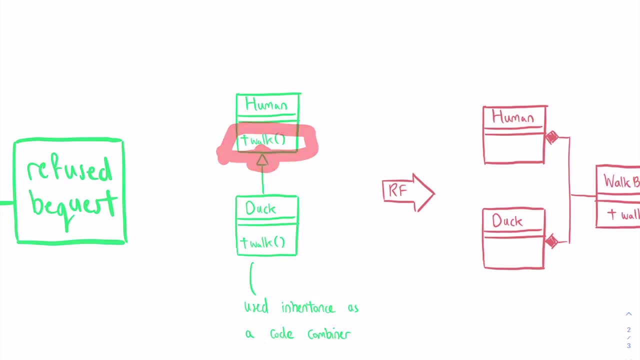 just inherit the magical creed andählt the same way, right, um. but we also have to do that in order to inherit from the same code the method here in human to allow for the duck to walk. let's say it's. you know, it's a pixelated, like old school type of game that walk really just means you. 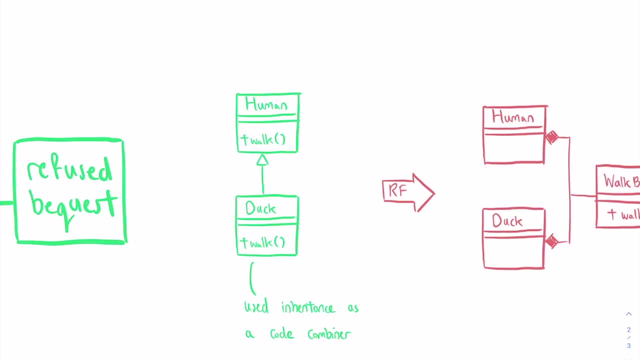 change the position from this to that, okay, and activate the animation of the: the walk sprite for duck and walk, or walk sprite for human. so it's the same code, so why not? we just inherit it. but you know, uh, it's wrong. okay, because, uh, what are you doing here is that you're trying to. 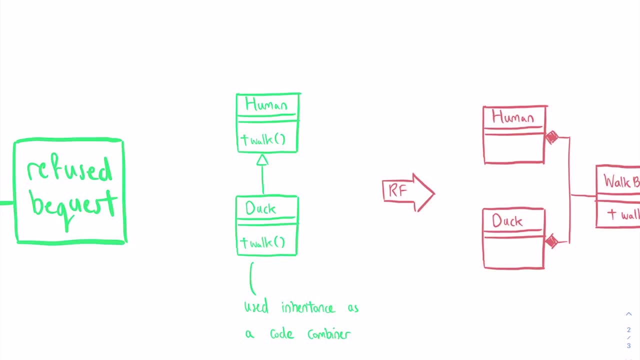 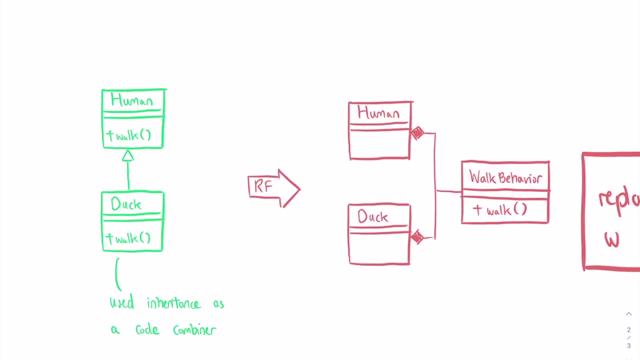 use inheritance as a code combiner. in essence, you know you're you are along the right line of trying to reduce duplication of code, uh, and you know, trying to, uh, just make your architecture, um, or your code pattern a bit nicer, okay, but this is the wrong way because, firstly, you know, 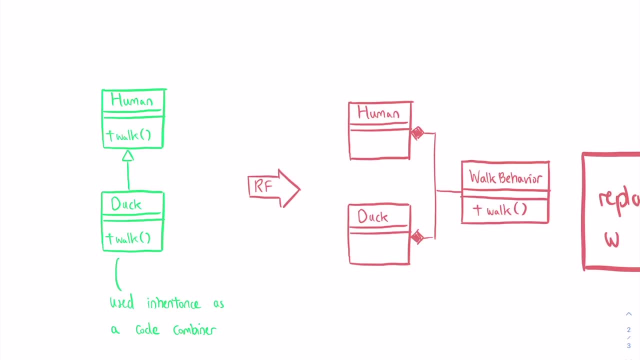 a duck is really not a human. yeah, and when you the concept is different, most likely in the human you already would have other uh functions that you know are not uh cannot be done by the or are different from the duck, like, for example, just now that uh talk, okay, or maybe i'll just draw it in here, okay, since it is part. 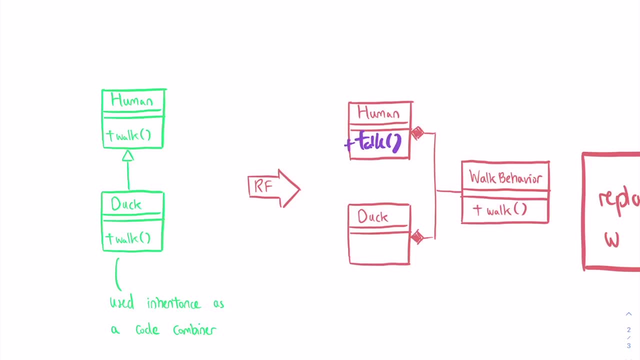 of the human. okay, so this talk method, um of the human, uh, most likely it would be different from that. or rather, you know, let's say, in this example, human has a talk function and the dog has the duck is another talk, or there's no talk, the duck has only can quack right, and it's entirely different. okay, let's say 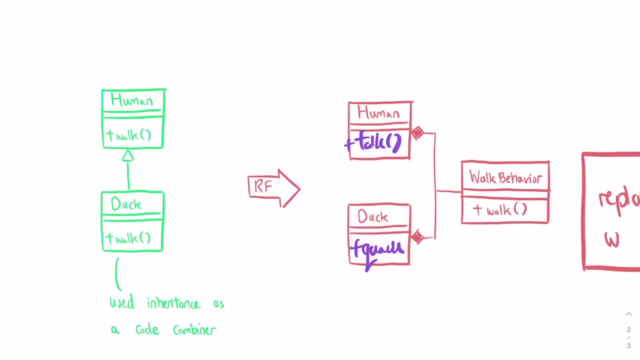 the implementation is entirely different. so here already there's a conflict. so therefore, uh, you know, we should change the relationship, okay. and since we understand, we know that walk is, you know, the same code, okay, so therefore we can uh sort of extract this walk method into another type of a class, you know called the behavior class or walk behavior. 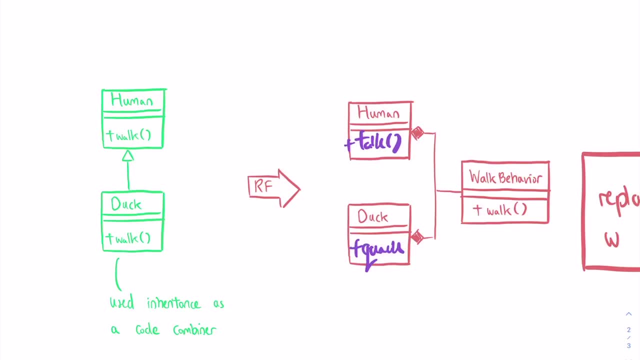 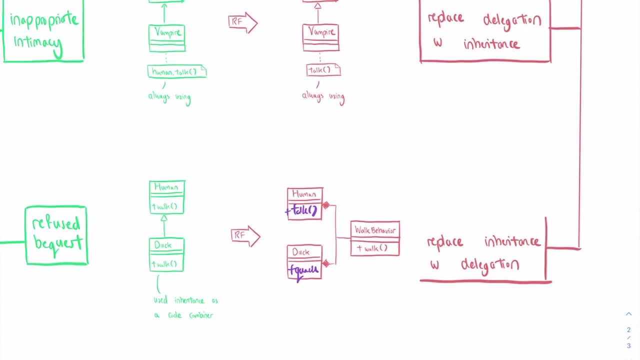 class, to be specific here, okay, which can be uh, composed, you know, uh, or contained inside both the human and the duck right, using a composition relationship. okay, so this in the reverse way, we are trying to replace um delegation, oh sorry, replace inheritance with delegation, all right, so these are all examples um that you can find from many uh popular websites, you know. 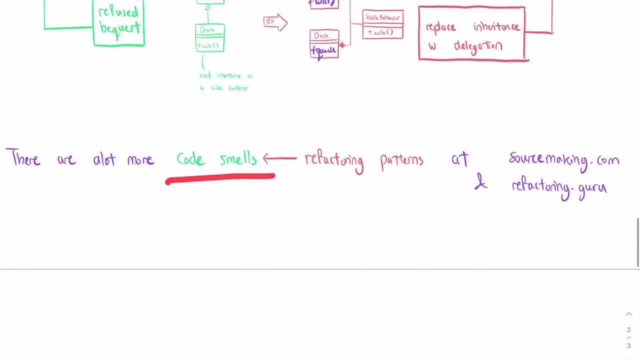 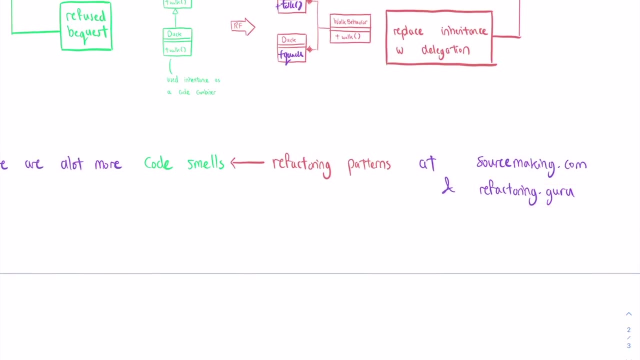 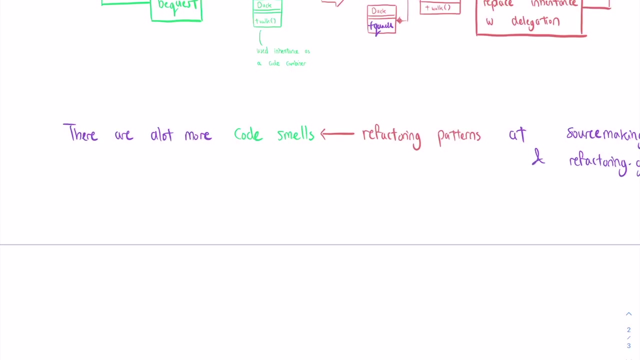 you can find a lot more code smells from you know websites like sourcemaking or refactoring, just like how design patterns you know help you figure out the right code structures before you you code right refactoring patterns actually help you figure out- sorry, figure out the. 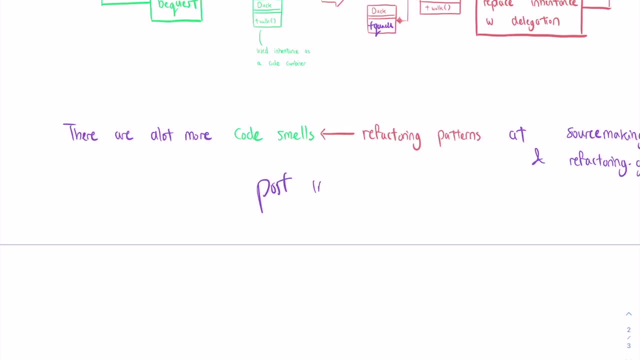 write code structures post implementation, So after you code. that's why it's a maintenance phase. Before the maintenance phase, it's a design phase. for example, Design patterns help you understand what you need to do before you code or guide you along the right way before you code or